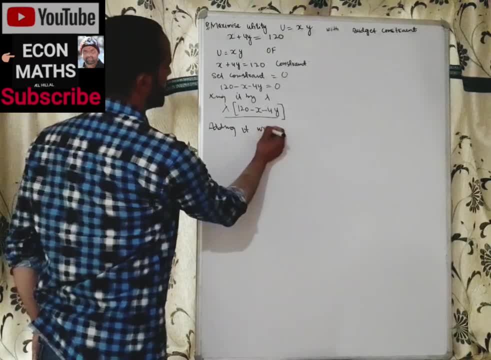 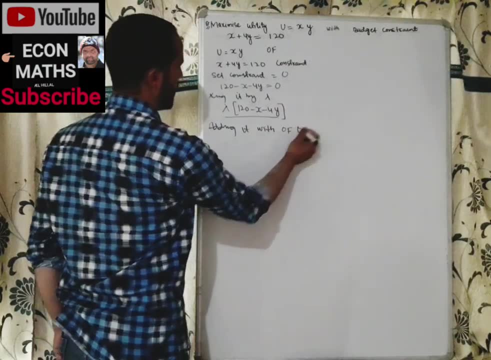 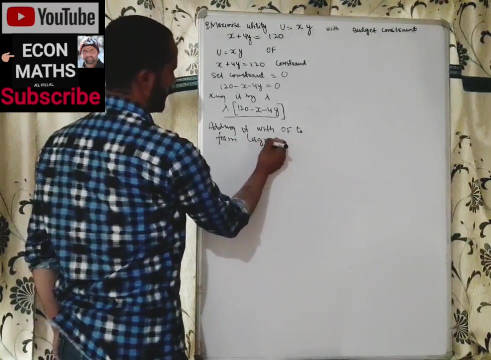 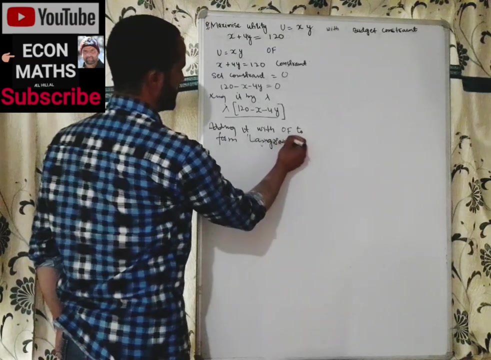 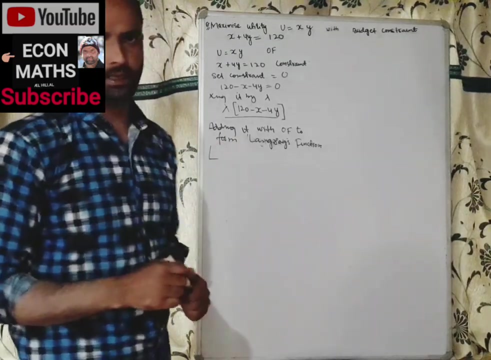 that with the feature And the function will become bye, And then X prime will become x prime. So thanks forbak род class, Bye, Bye. minus. the lagrangian function is equal to: and that is objective function, that is uh x into y. 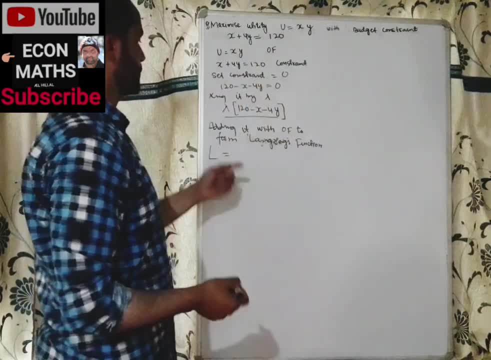 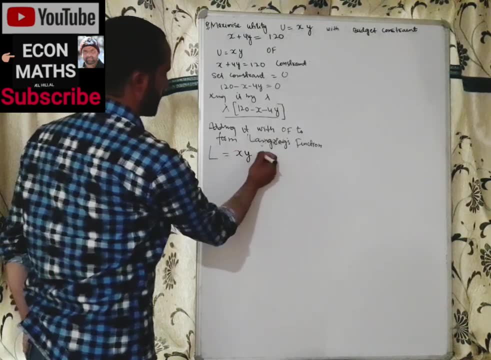 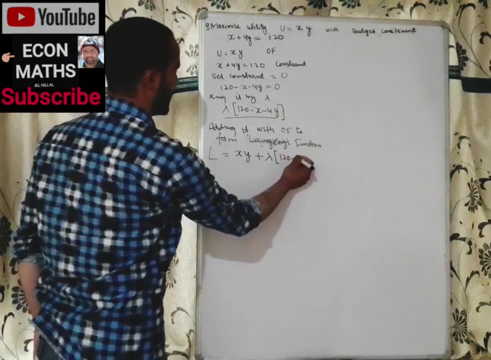 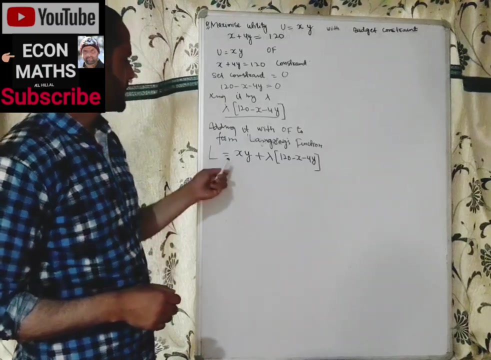 plus this constraint. so i will add these two terms to form the lagrangian constraint. so this is our objective function. is x into y plus- now i will add this term with this. so this is lambda into 120 minus x minus 4 y. now this is our lagrangian function. now to get the optimal. 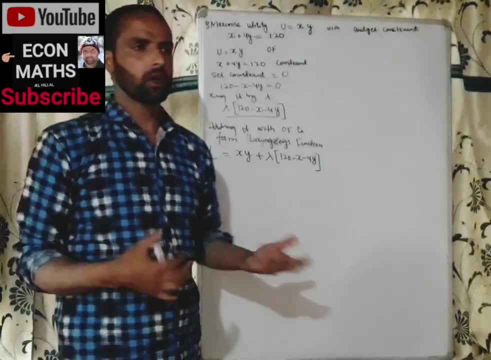 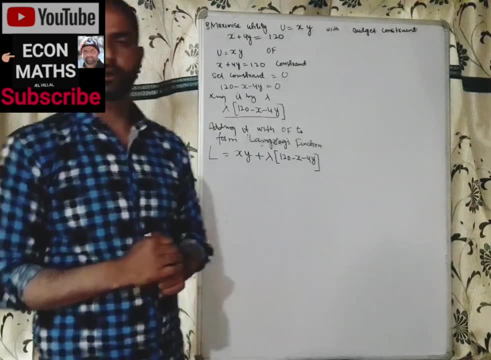 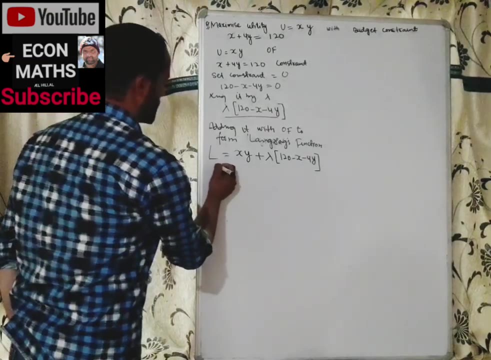 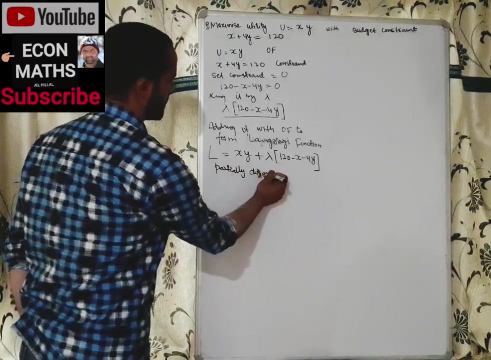 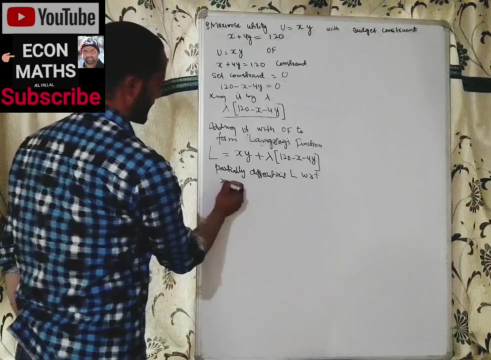 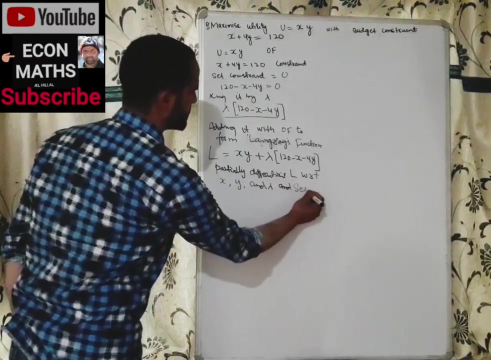 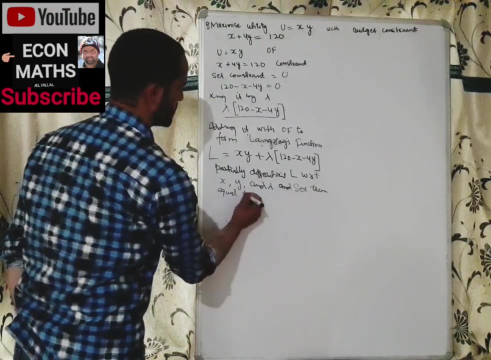 value of x, y and lambda. i have to, or we have to, partially differentiate this lagrangian function with respect to x, y and lambda and set them equal to zero to get the optimal values of x, y and lambda. so i will write here partially, partially differentiate l with respect to x, y and lambda and set them, set them equal to, equal to zero. 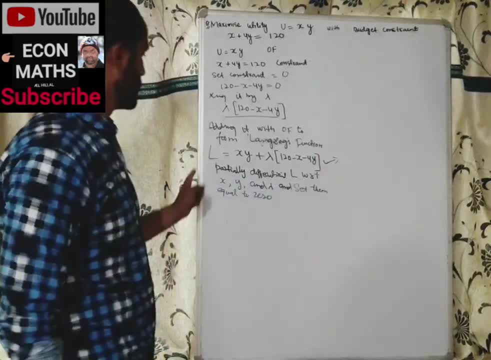 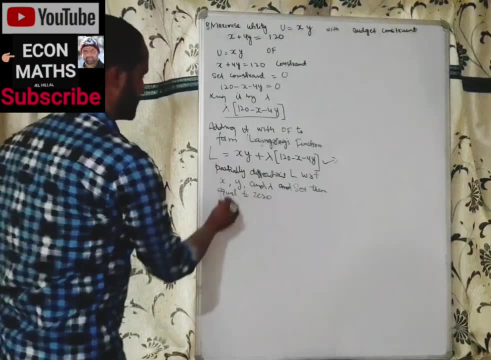 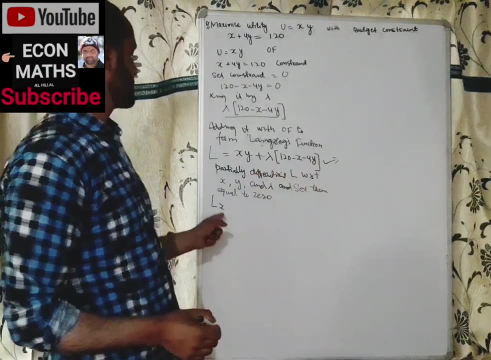 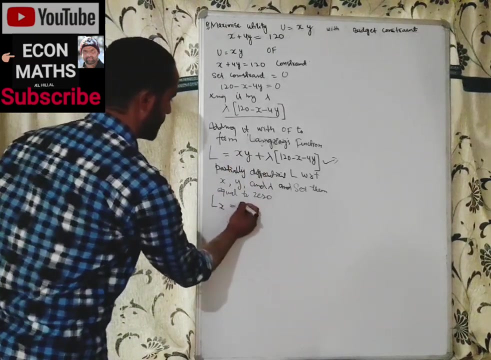 now i will differentiate this lagrangian function with respect to x, y and lambda to get the values of these variables. now l of x. now this l of x means partially differentiating this equation with respect to x. so this will become: now here x into y. the derivative of x is 1, so here it is y, plus now here lambda, into 120. so 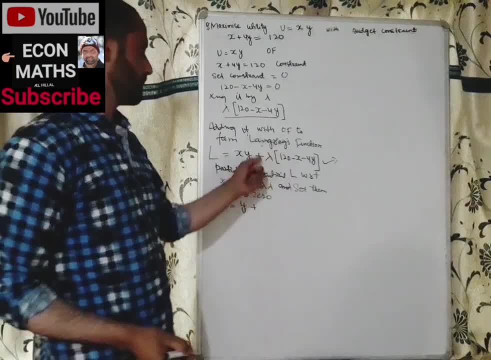 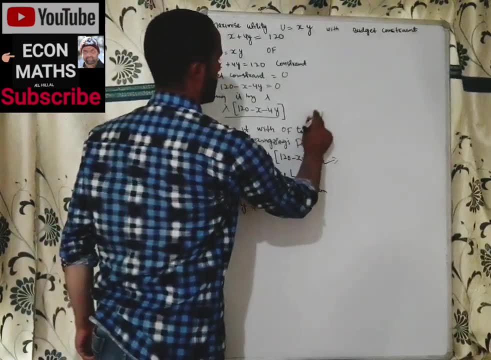 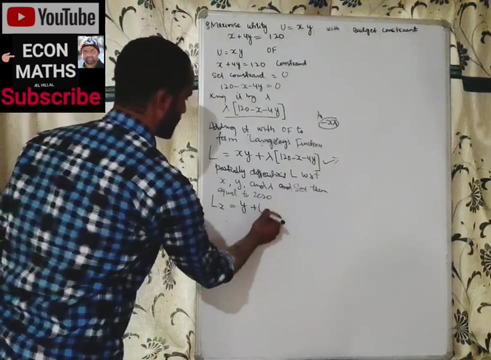 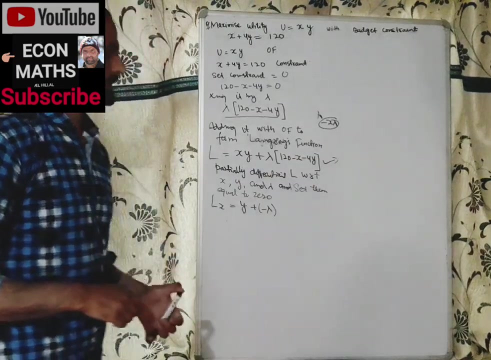 no, y x is um here, so it will become zero. now lambda into minus x, lambda into minus x. it is here minus x lambda. its derivative is minus lambda here. so i will write here: minus lambda, now lambda into 4, into y. so no, y x is uh involved here, so it is derivative is 0.. now i will set this: 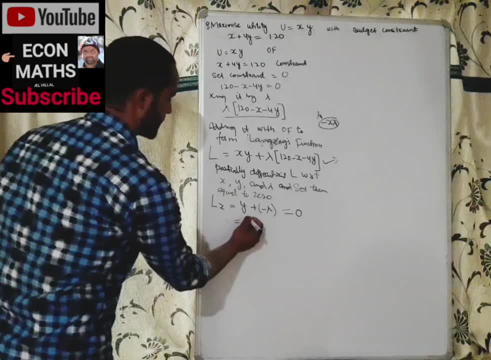 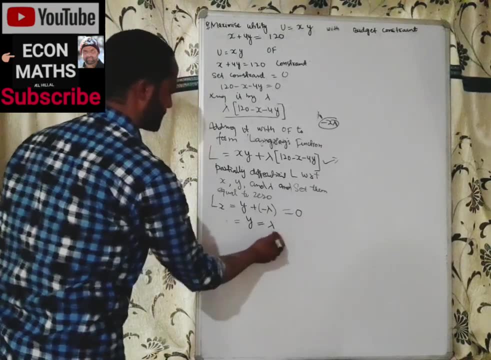 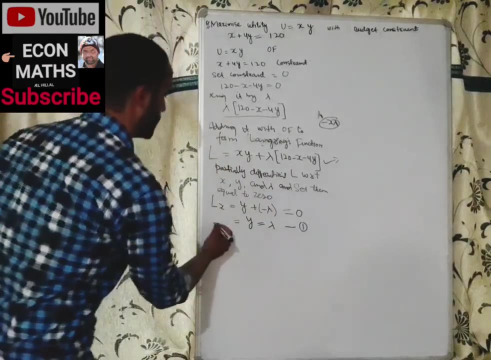 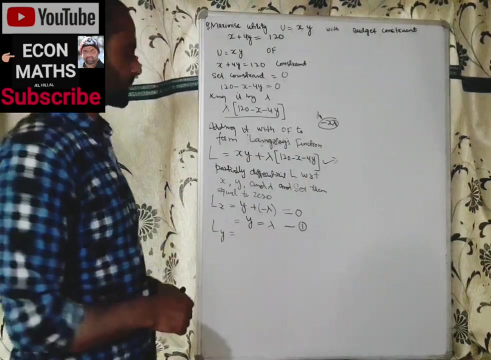 equation equal to zero, or this will become: y is equal to. now, transposing this to rhs, this will become plus lambda. let's be equation first. similarly, i will differentiate this with respect to y. now l of y, minus, partially differentiating this lagrangian function with respect to y. so this will become: 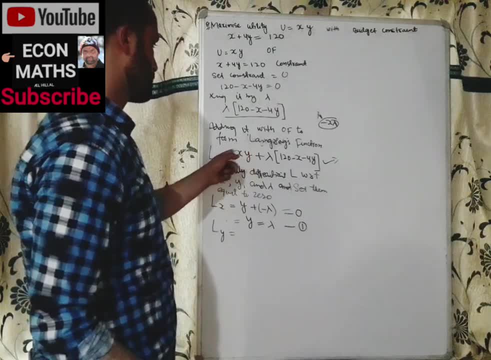 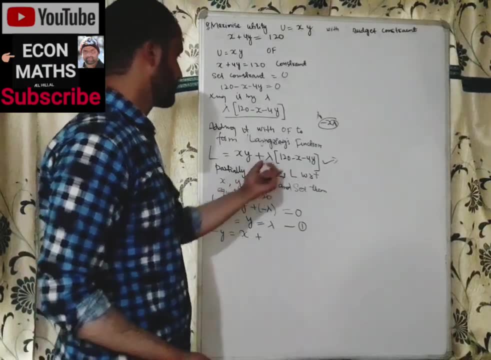 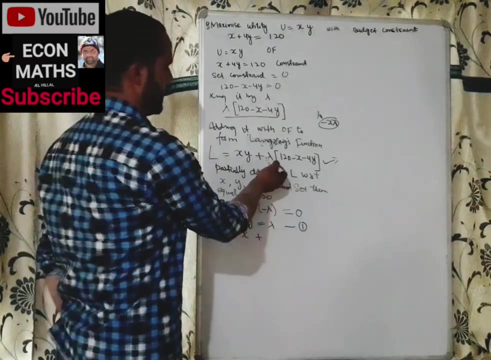 here x into i, y. now the derivative of y is 1, so here it is x plus. now here lambda into 120, no y involved, so it is 0, plus lambda into minus x, no y involved, so the derivative is 0, and lambda into minus 4 into y. now this will become minus 4 y, lambda. 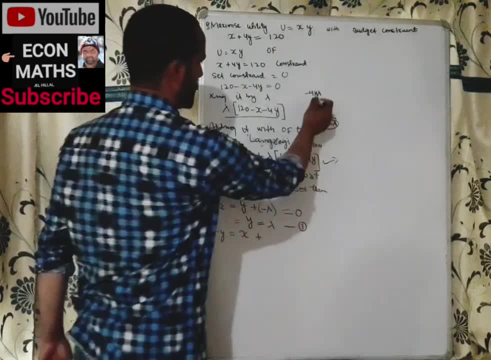 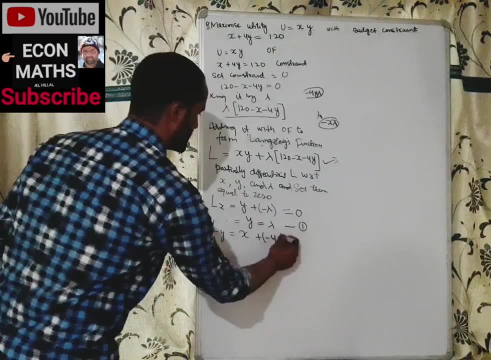 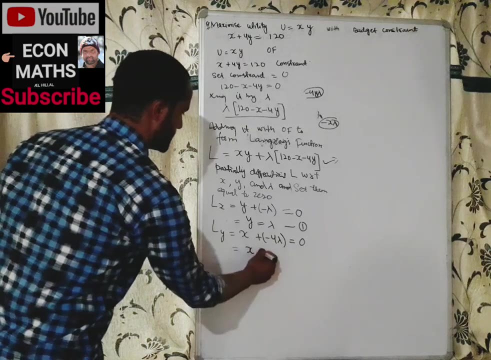 minus 4 y lambda. now the derivative of this with respect to y is minus 4 lambda. so i will write minus 4 lambda and set it equal to 0.. now solving this will become x is equal to transposing this to our h. s will make it. 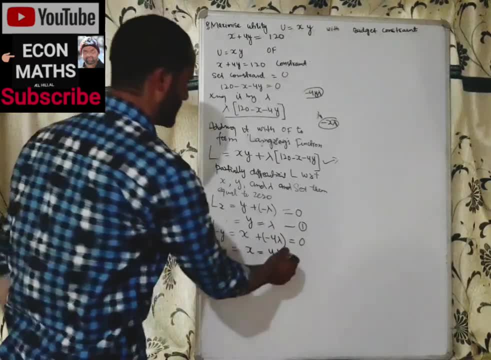 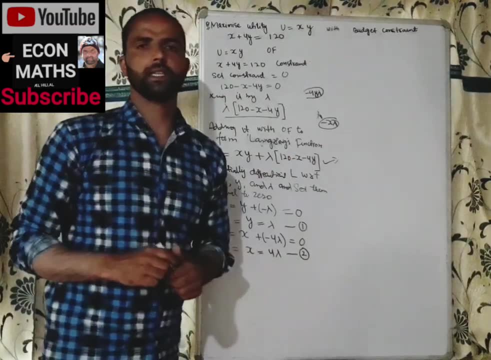 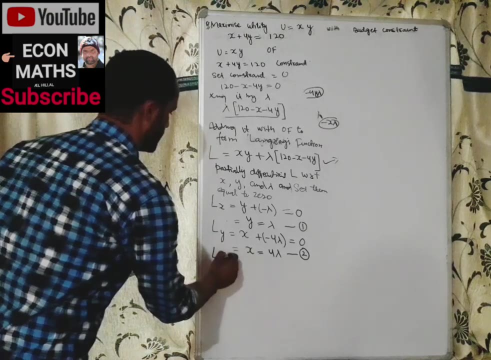 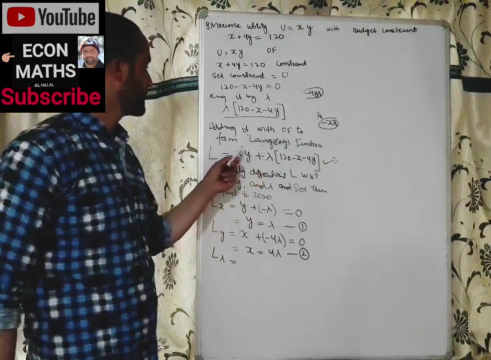 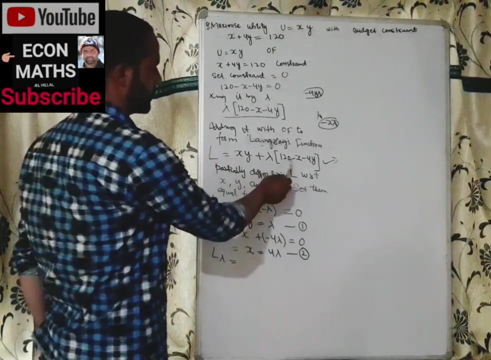 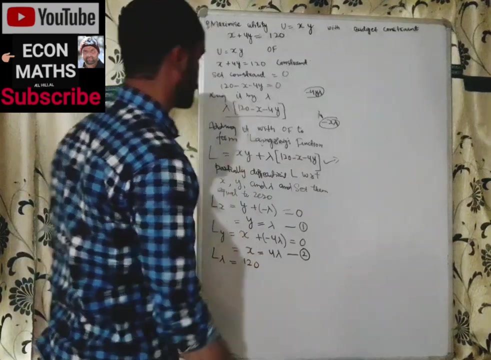 plus 4 lambda. now let this be equation second. now, in the same way, we have to differentiate this equation with respect to lambda. partially, that is obvious. now l of lambda is equal to now. Now differentiating this with respect to lambda minus here, x into y. no lambda is available here, So its derivative is 0.. Now lambda into 120 will become 120. Now lambda into minus x. So this will become minus x and lambda into minus 4y. 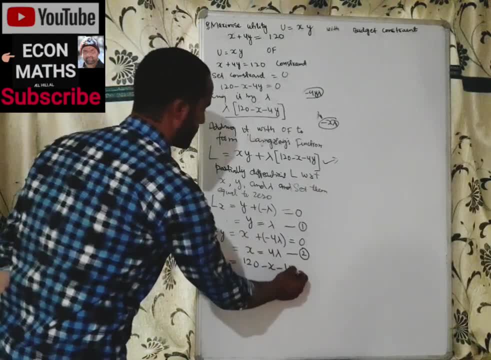 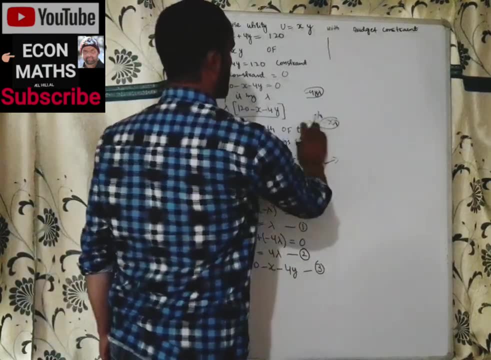 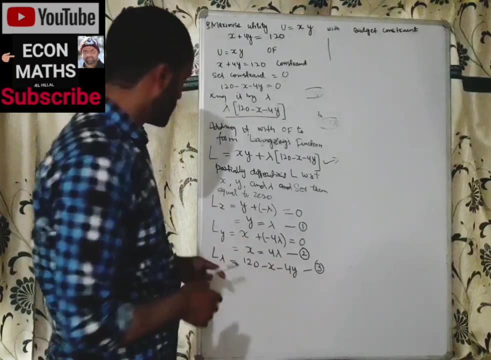 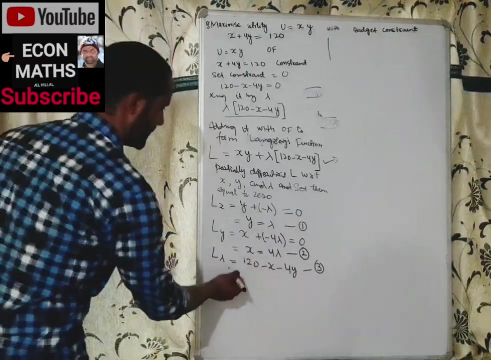 So this will become minus 4y. That is the equation. third, Now to get the value of x and y here we will divide equation 2 by 1. Or I will write. so I will write here this dividing equation. 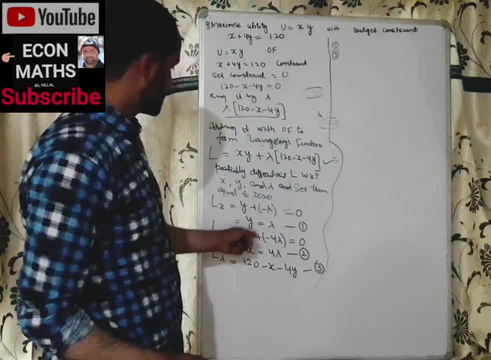 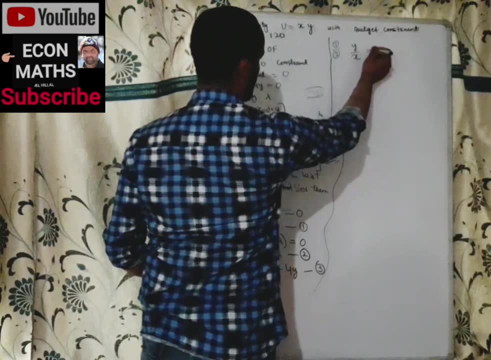 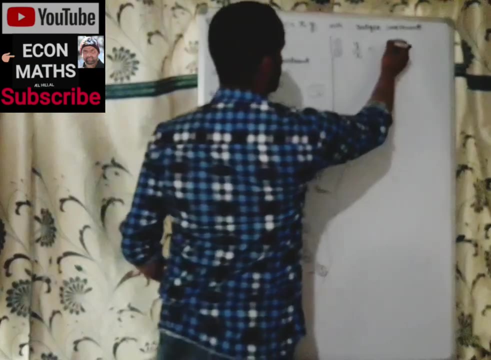 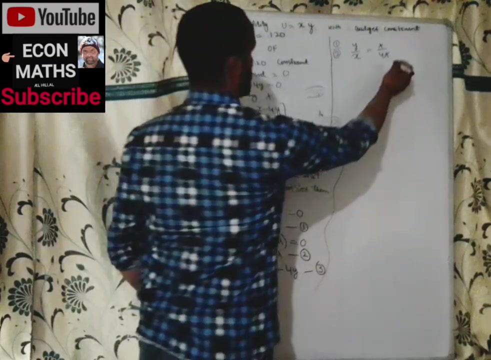 First and second. So this will become y over x. implies y over x is equal to: now lambda into sorry lambda divided by 4 lambda, That is, lambda over 4 lambda. Now lambda lambda will cancel out. This will become 1 over 1 over 4.. 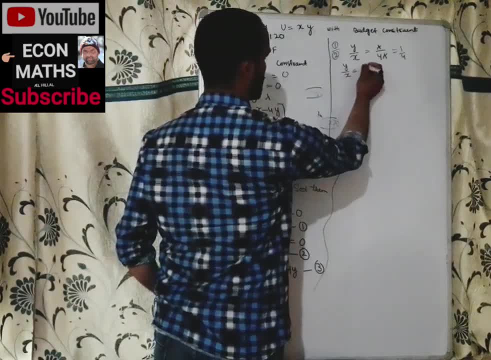 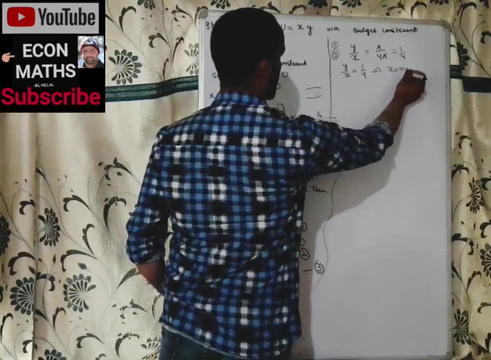 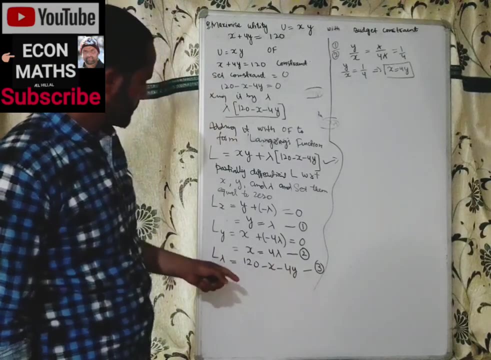 Now this is y. Y over x is equal to 1 over 4 implies 4y, or x is equal to x is equal to 4y. Now I will put the value of x is equal to 4y in the third equation to get the value of y. 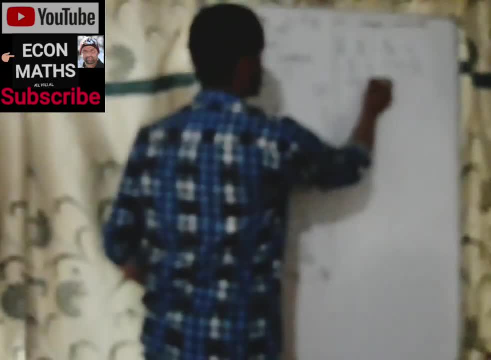 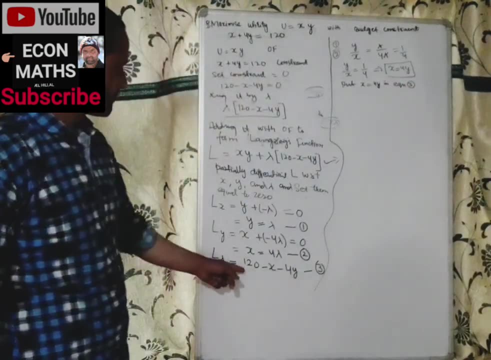 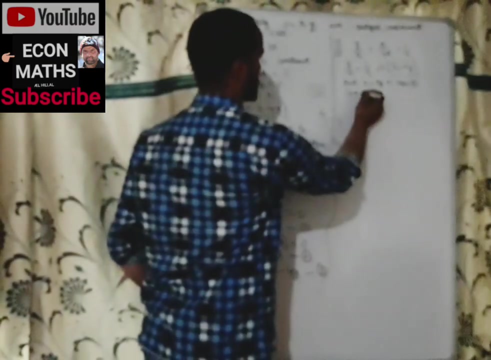 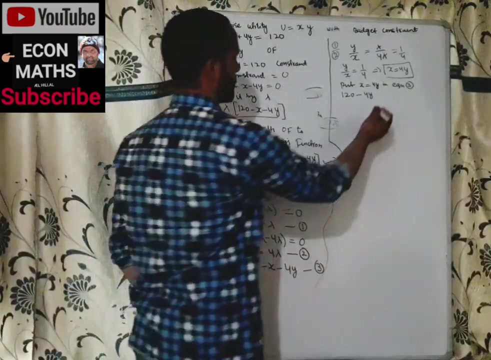 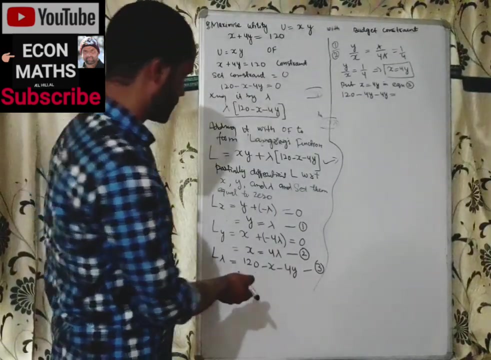 So I will put x is equal to 4y in equation. third: Now I will put this here in this equation: So this will become 120 minus now the value of x is 4y, So I will write 4y, And here is minus 4y Minus 4y is equal to sorry, here it is. I have to set it equal to 0. 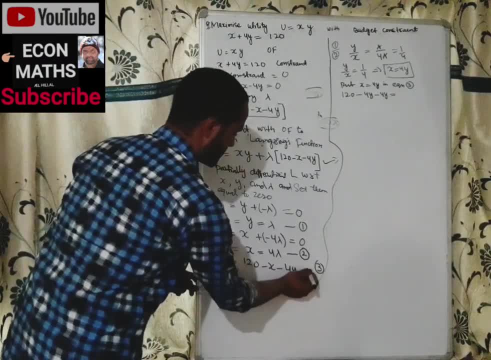 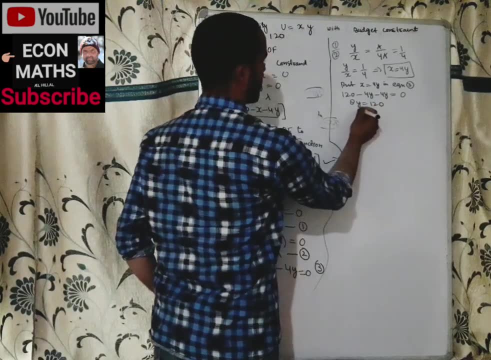 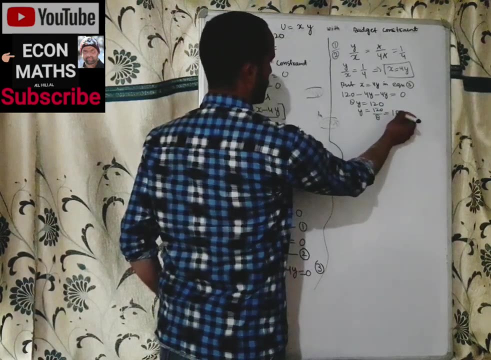 So this is 0.. So this will become 0. Or I will write at: y is equal to 1, 20, or y is equal to 120 over 8.. So this will be at: 1 is our and this will be at: 5 is our. So y is equal to 15.. 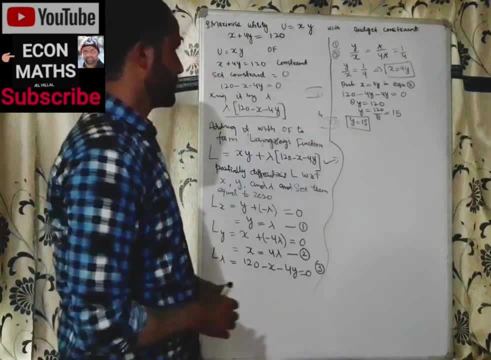 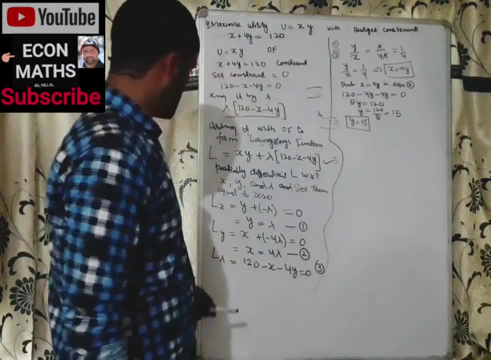 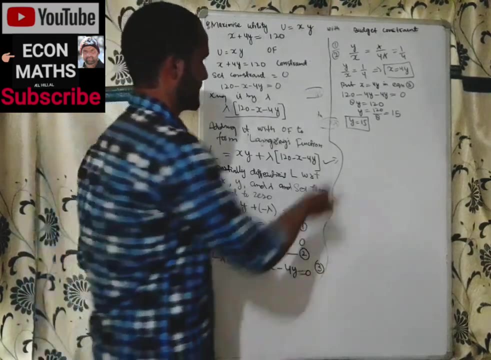 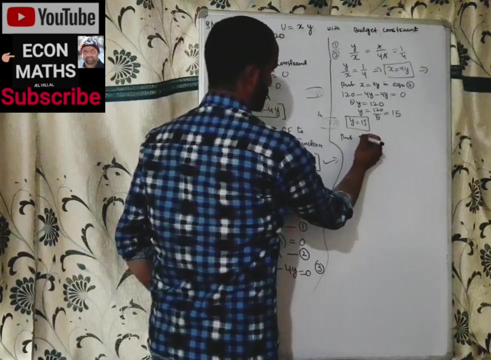 Now y is equal to 15.. We have to find the value of x. Now I can put the value of y here Or in this equation to get the value of x. So I will put this here. Therefore, put y is equal to 15 in this equation. 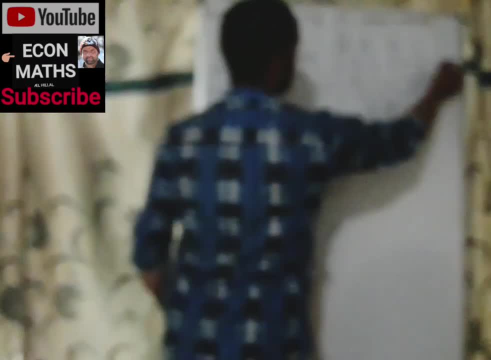 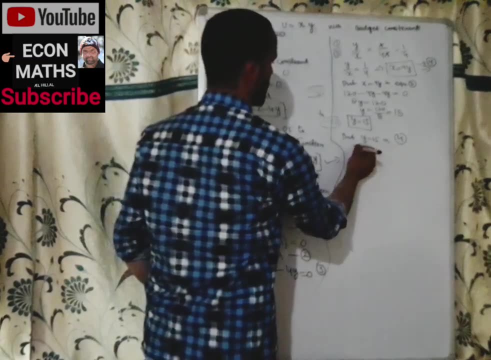 Let this be something. it is 4 here. Let this be equation: 4 in 4.. So this will become x. So x is equal to now 4 into y. This is 4 into 15 is equal to 60.. 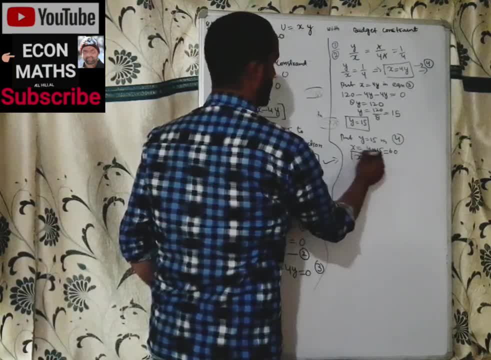 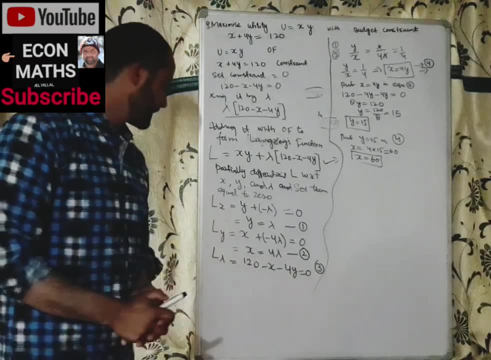 So x is equal to 60.. Now we have got the value of x and y. We have to find the value of lambda. Now, to get the value of lambda, we have to see in which equation the lambda is available. 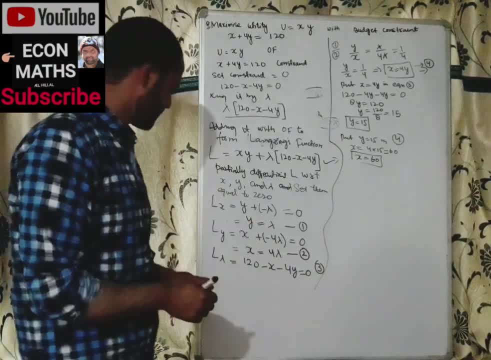 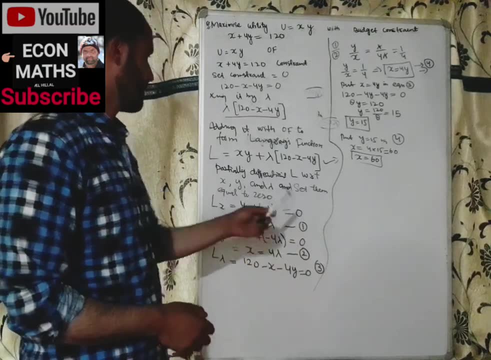 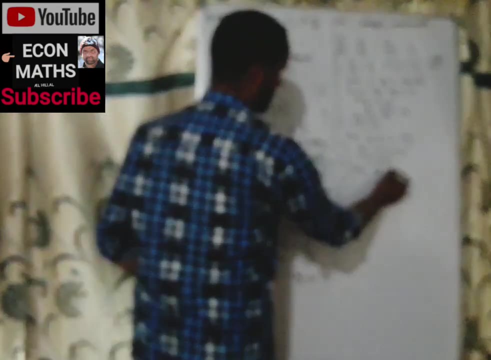 So I will put the value of x or y or both in either of the two equations. So I will put the value of x or y or both in either of the two equations. So I will put in this equation Now, put y is equal to 15 in equation first: 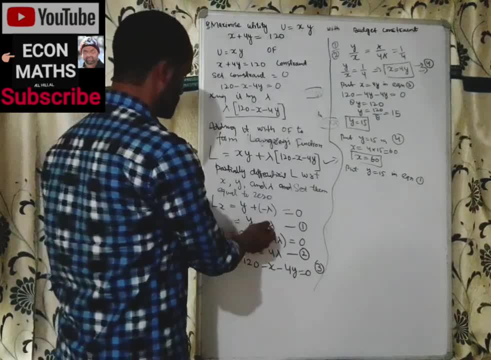 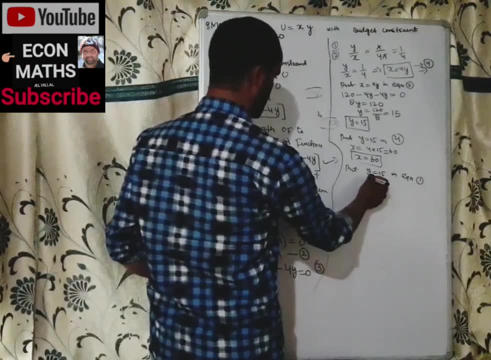 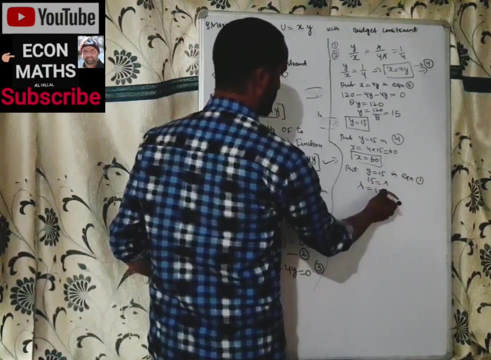 Now, this is our first equation, So I will write here This will become y In place of y. I will write: 15 is equal to lambda, So the value of lambda is 15.. Now I have got the value of x, y and lambda. 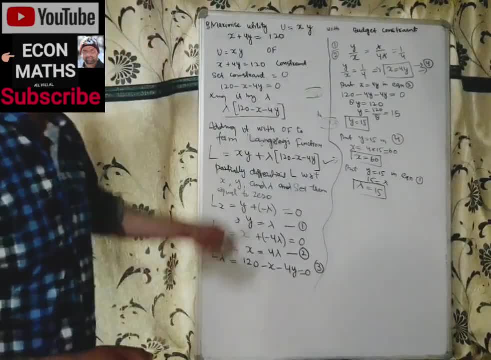 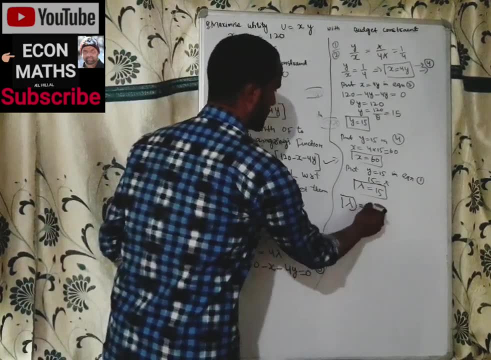 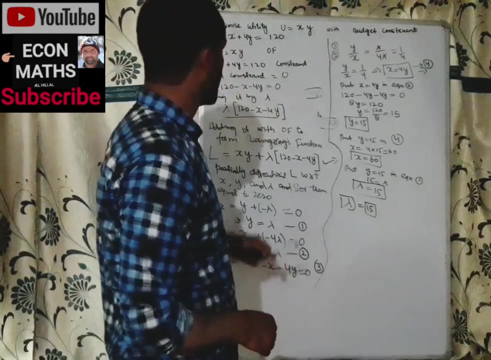 These are the optimal values of the variables which we have calculated here. Now, what does this lambda mean? Lambda is equal to 15.. What does this signify? Now, this lambda tells us? this lambda tells us, if there is incremental change, one unit change in the constant of the constant. 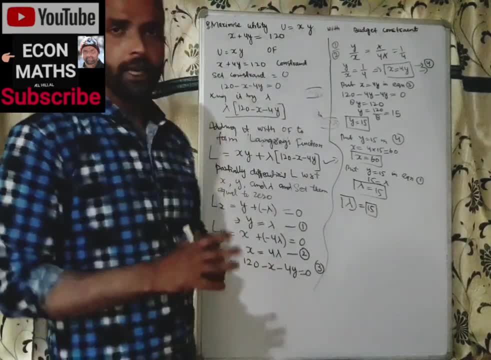 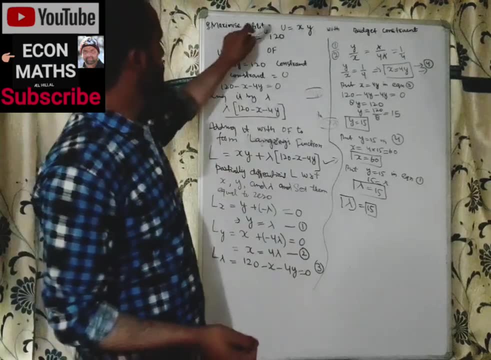 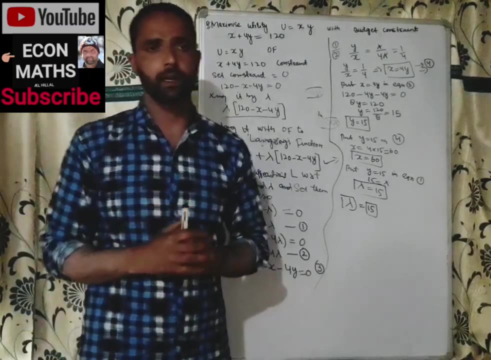 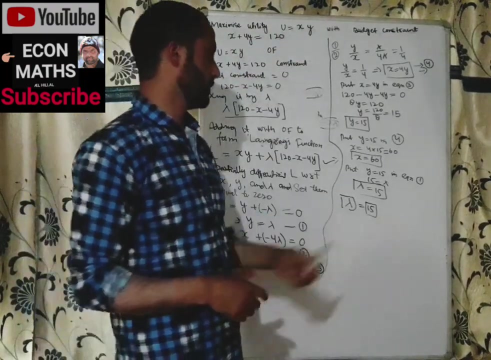 This is the constant. of this constant, If the- or I can say, if the budget increases by one unit, this objective function will increase by 15 units. Or I can say: if there is one unit change in the constant of the constant, the objective function will change by 15 units.